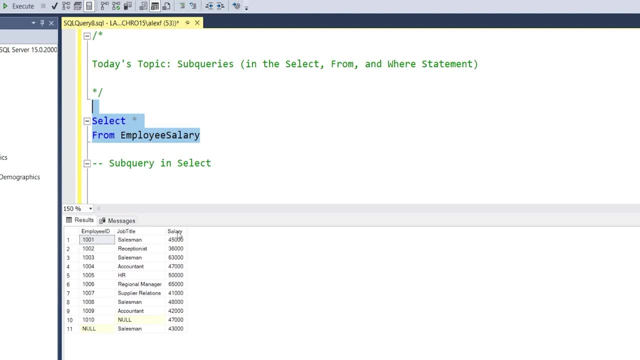 So we have an employee ID, we have a job title and then we have a salary. So, really quick, I'm going to show you what it looks like to have a subquery in the select statement. So let's go down here really quick, And what we're going to try to do is kind of do something like a Windows. 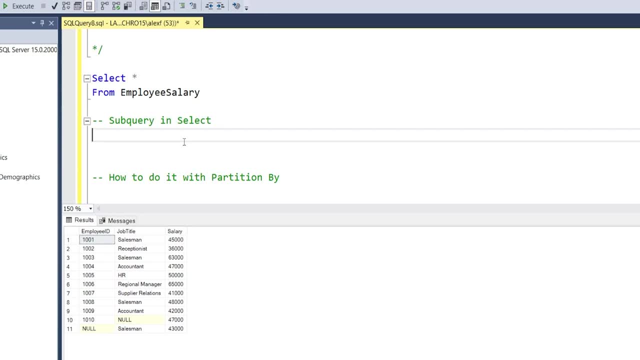 function, but without actually having to do the Windows function, And so we're going to do this with a subquery. So I'm going to select and really quick actually, let me copy this: So we're going to do employee ID. There we go, We're going to do salary And now we're going to start. 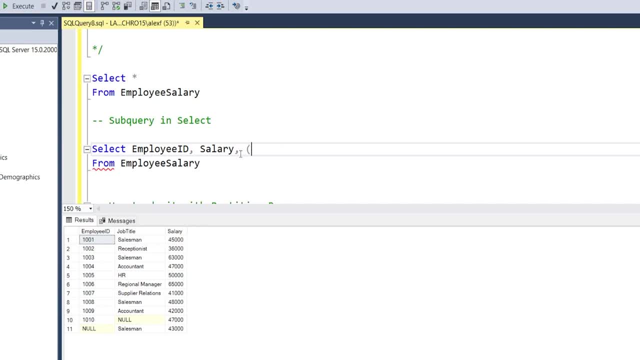 building our subquery, So we need to do an open parentheses- And I'm just going to copy this really quick because we're going to be doing it off of that table. So we're going to say select and then I'll paste that and close it as well. But what we want to do is we want to say average. 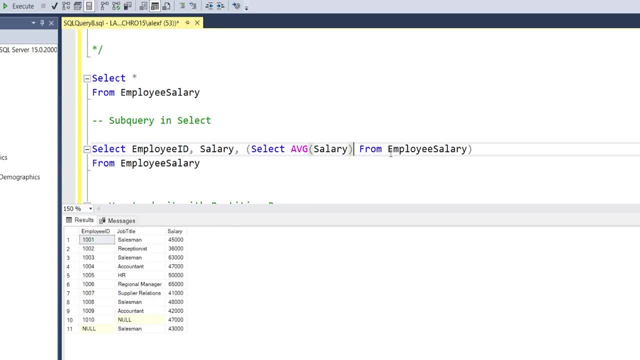 and salary. Now, what this is going to do is it is literally going to run this, and let's run this really quick. It is going to run this and it's going to show that the average salary for all the employees is $47,900. 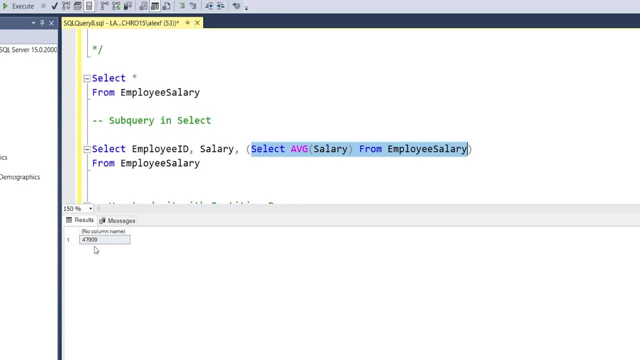 So we are looking at the average salary for every employee. So when we run this, it is going to give us the employee ID, the salary, and then, in the very last one, is going to show the average salary for every employee. Now it doesn't have a column header, so, or column name, So let's give it, let's. 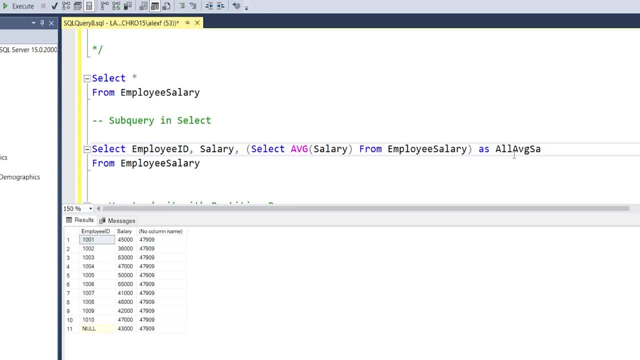 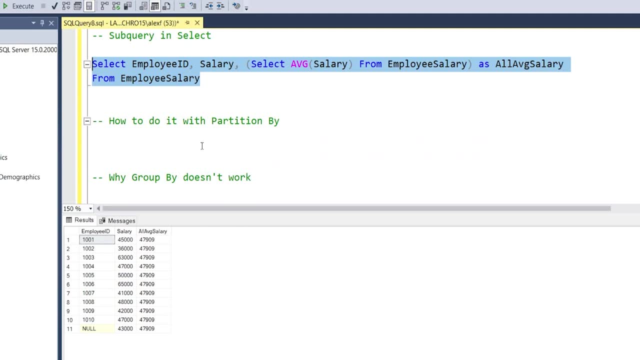 say as all average salary, And we'll run that one more time, just make it look a little prettier. And we can also do this in partition by. I'm going to super quickly, just really quickly, write this out- it should take no time at all- And then I'm going to show you why we can't do this without the 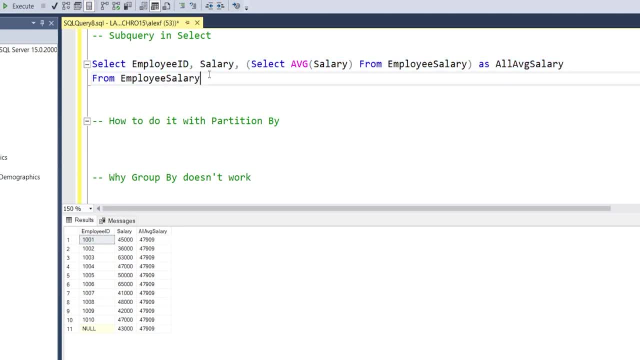 sub query why you aren't able to do this with a group by so really quickly. let me copy this. I'm gonna put it right down here And we're going to say: average salary: whoops, And we can get rid of all this. And we're gonna say over, and we're not going to partition it by anything, But let's run. 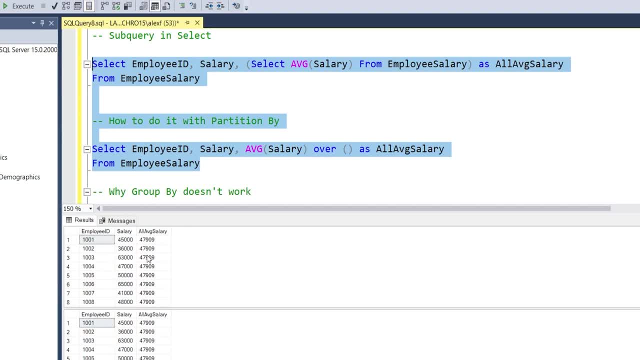 both of these at the same time. you'll see that they're the exact same outputs And so it's just a different way of doing it in this example. But it really is just to show a comparison of how you might be able to use a sub query in the select statement. Now you might be wondering why group. 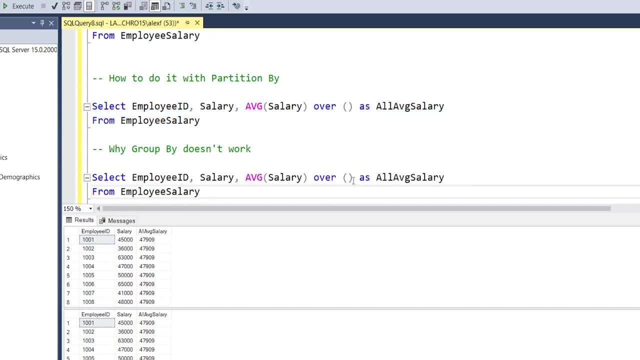 by does not work for this really quickly. I'm going to write this out And let's get rid of that. And we'll say group by- whoops, let me at least try to write it correctly. Group by, and we'll do. employee ID. 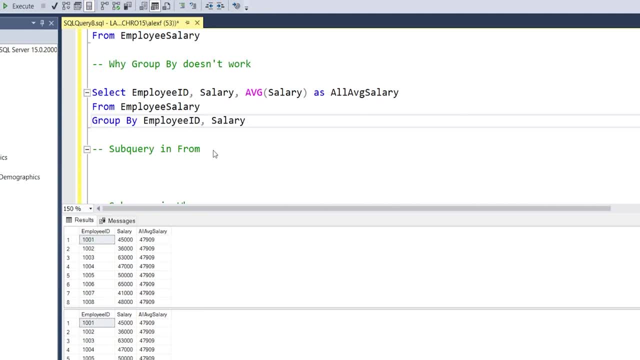 And we also have to do salary, And then we'll say order by 12.. So let's run this And, as you can see, since we have to use the group by groups, by both the order ID and the salary, and so we're not. 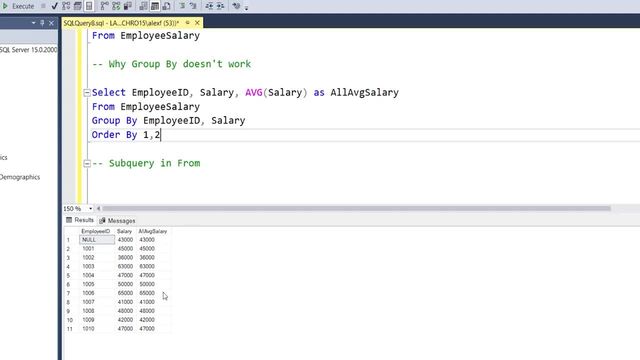 going to be able to get that all average salary that we're looking for, that we can get in the partition by and also the sub query in the select statement. Now I'm going to show you the sub query in the from statement. So let's just get rid of that really quick And let's say select everything. Let's say from and we're 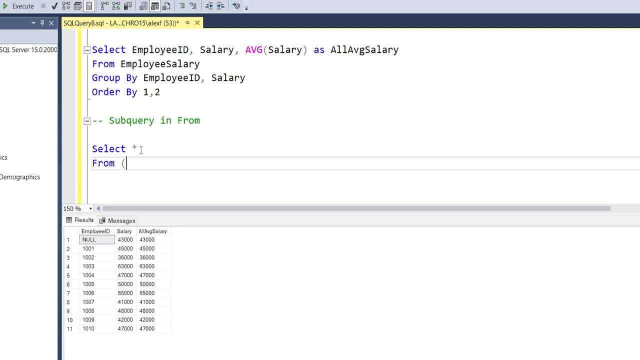 going to do an open parentheses here, And here's where we're going to write our sub query. So if you have watched previous videos where I've done tutorials on the CTE or tutorial on the temp tables, this is one that is very much like those, except, I think, a little bit less efficient When 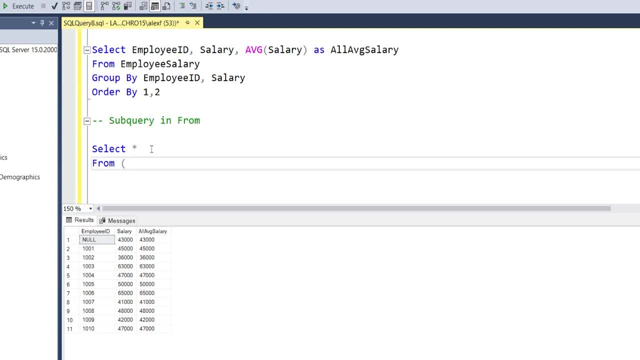 I'm doing something where I'm creating a table and then querying off of it, which is what we're about to do. I much prefer a CTE or a temp table- sub queries tend to be a little bit slow- compared to a temp table or a CTE. I tend to use temp tables a lot more because you can reuse them over and over. 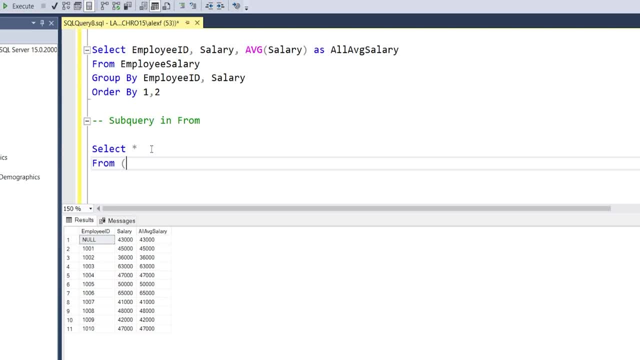 whereas a sub query? you cannot. you have to write it out each time. So, really quickly, I'm going to show you how it's done, Although I don't really recommend using this method. Really quickly, let's go up here and let's steal this partition by really quick. This will be our sub query. 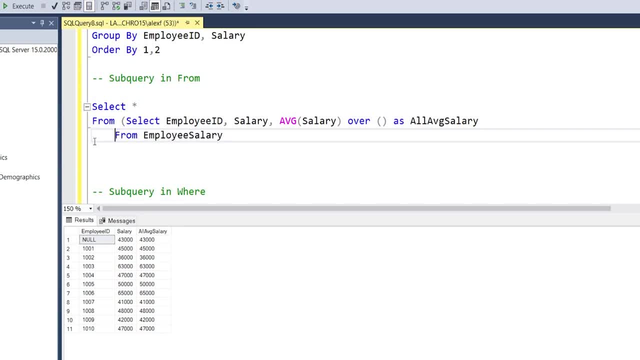 And let's paste this in here, make this look a little nicer So you can visualize it a little bit easier. So, really quick. what this is going to do is it is first going to run this and create this table again, much like a temp table or a CTE. So let's execute this really quick. It's going to. 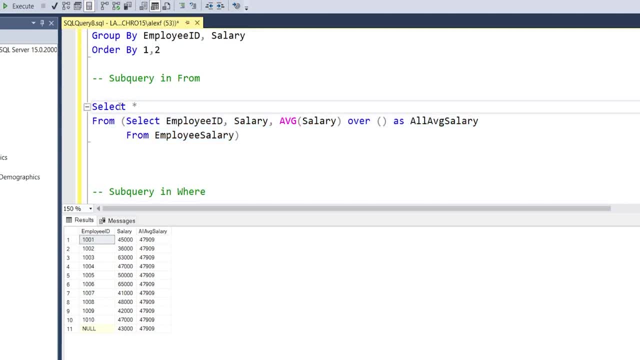 create this table and then it's going to allow us to query off of it. So I can actually say- and let me give kind of an alias to this- So I'm going to say temp table, dot, employee ID, And then let's say all average salary. So now I can. 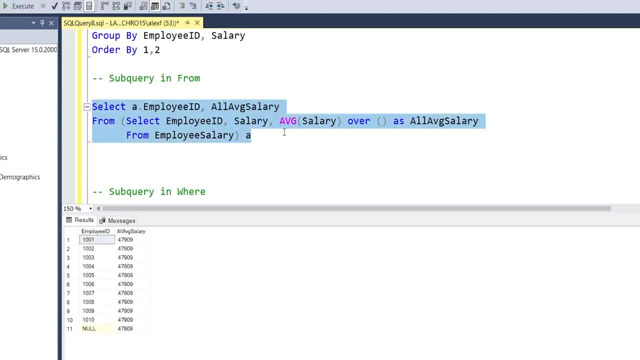 take columns from this inner query, if I want to, and just select those, or I can select everything and return that entire table Again. I much prefer a temp table or a CTE for this type of situation, But as an example I just wanted to show you how it works. Now let's go down to the sub query in the 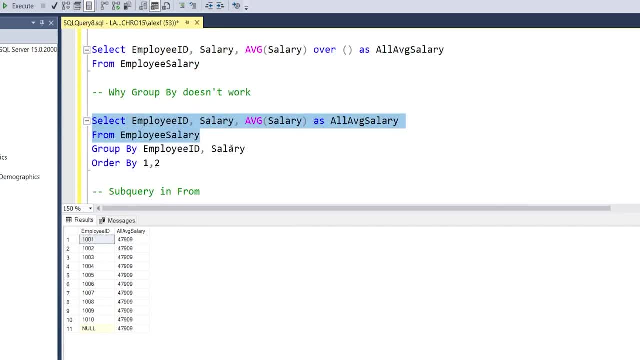 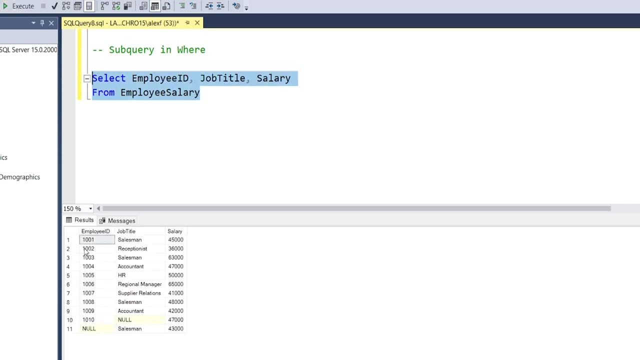 where statement. But really quick, I just want to steal this query So I don't have to rewrite everything, And let's get rid of this really quick and add back the job title. All right, let's look at this really quick. So we have our table that we've been using our employee ID, job title, salary. 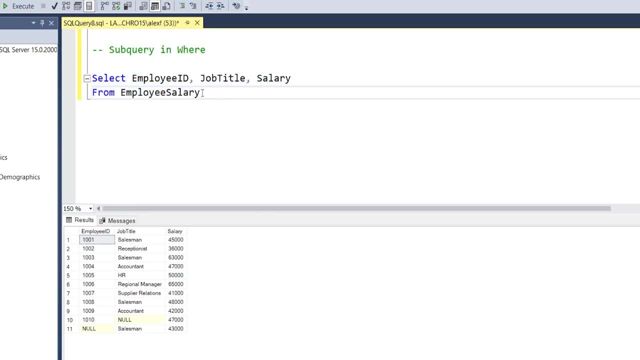 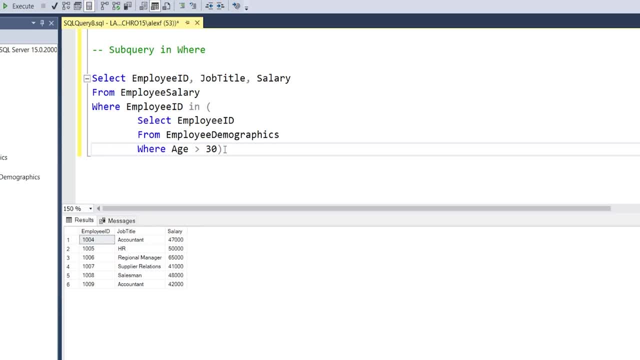 Now, if we wanted, we could join to that table and get a new job title. Now, if we wanted, we could join to that table and get a new job title and be a really good option in these scenarios. With that being said, this is the last video in the advanced SQL tutorials. 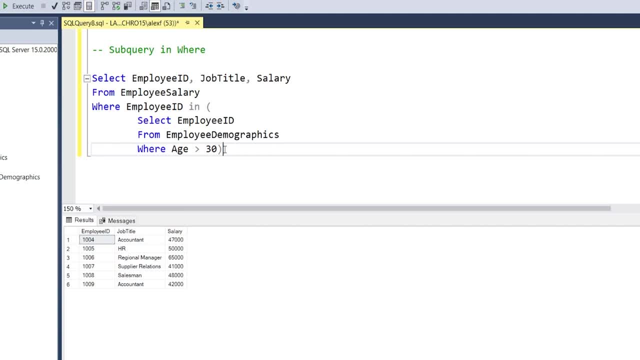 I hope that this series has been helpful and that you learned something along the way. Thank you so much for joining me. I really appreciate it. If you liked this video, be sure to like and subscribe below and I'll see you in the next video.